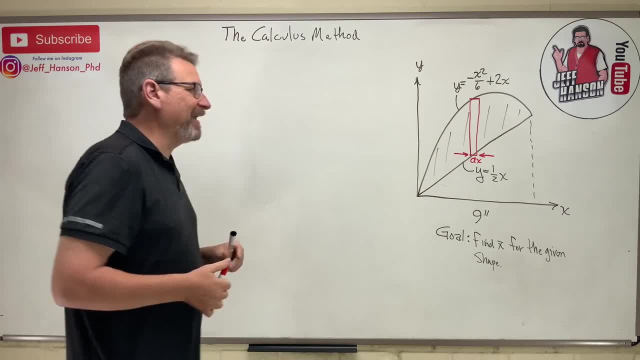 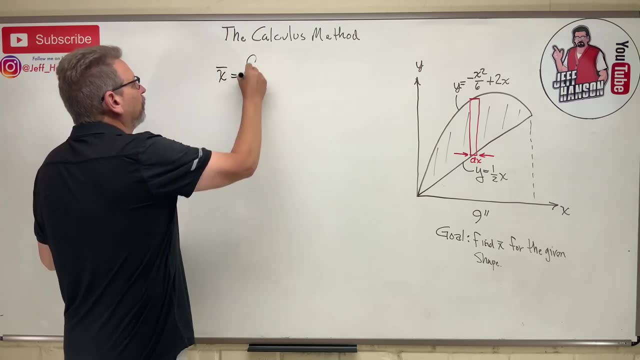 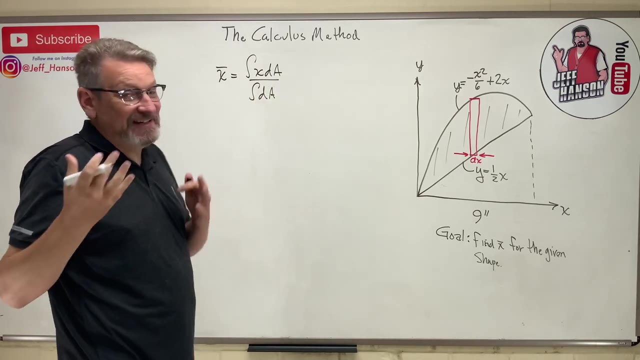 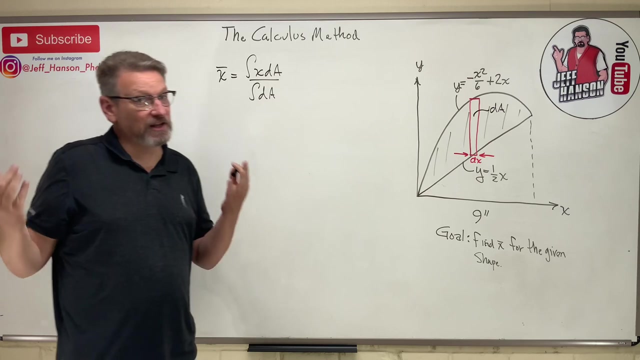 d, x, y, because that reminds me that you know, the equation for this is this: for x, bar is the integral of x, d a over the integral of d a, And we're talking about a differential area, and this rectangle is one differential area. Okay, and it isn't just that. 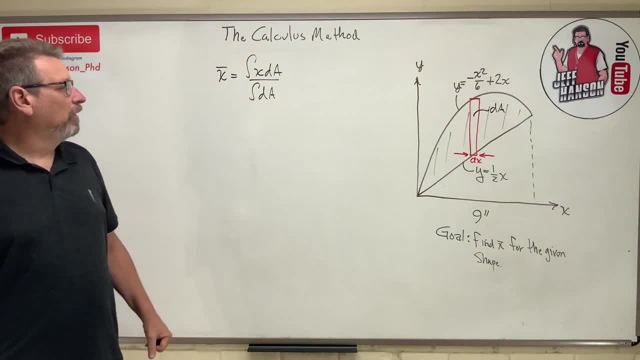 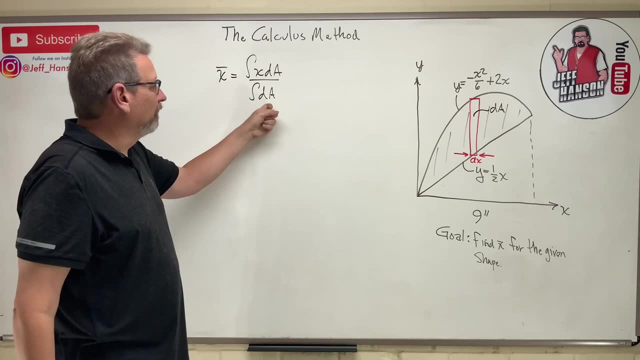 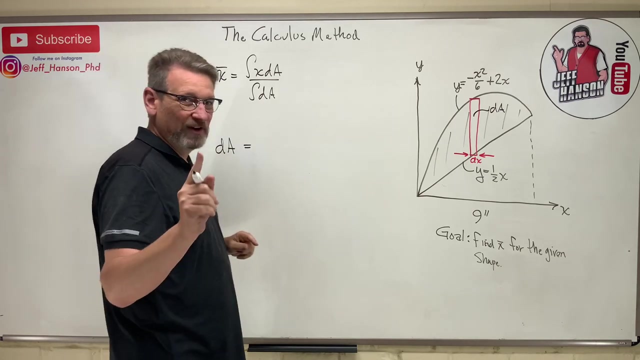 it's a rectangle, Okay. so when you do these problems, I suggest you start on the bottom with the differential area which is summing all of the differential areas up. Okay, so what is one differential area? One rectangle? It's just height times width, right? 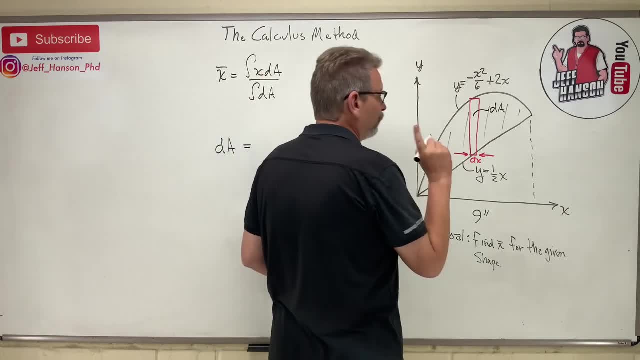 Well, the width, I already know, is d, x. So what is the height? And I'll draw you two arrows right. Here's one arrow, Okay, and here's another arrow. So what is the height of that guy? Well, 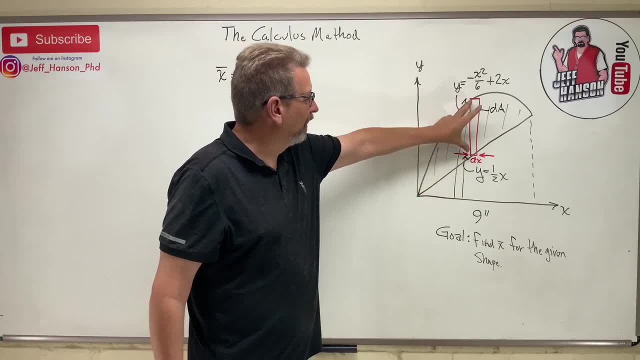 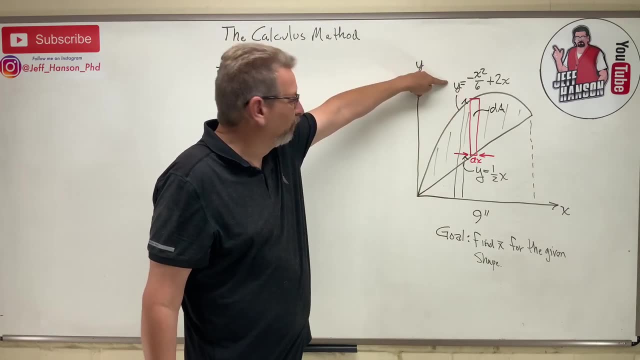 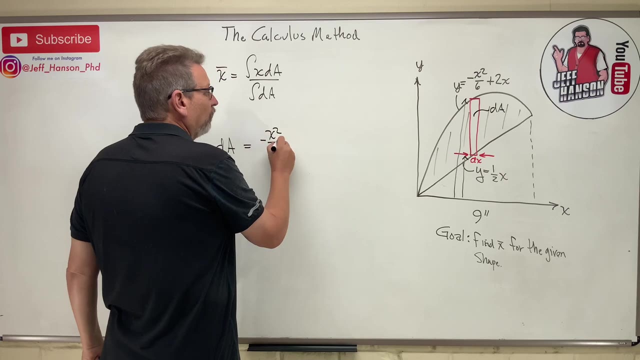 it's this whole thing minus this, and that would leave me with the height of the rectangle, isn't it? How tall is this? Well, that's how tall it is. They gave me an equation for all of the y values. So d a is equal to minus x, squared over 6 plus 2x. Okay, but from that I have. 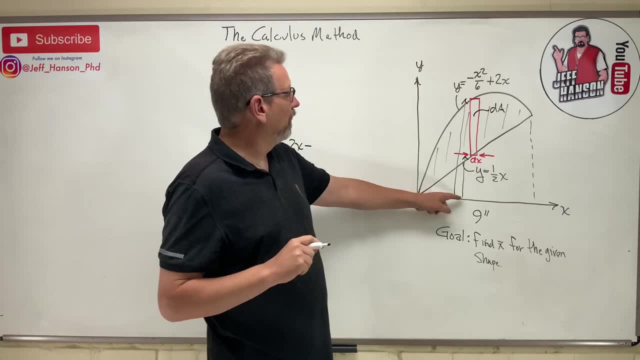 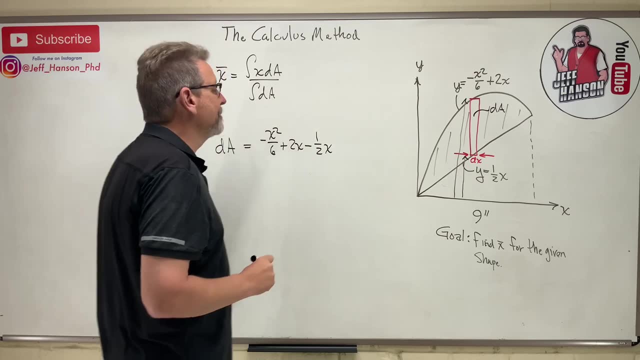 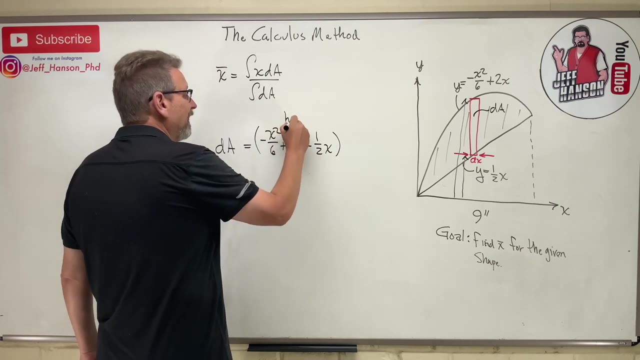 to subtract. What am I subtracting from that? Well, the y value on the bottom down here, which is one half x. Okay, Okay. So that's the height. This is the height of the rectangle, And then the width of the rectangle is. 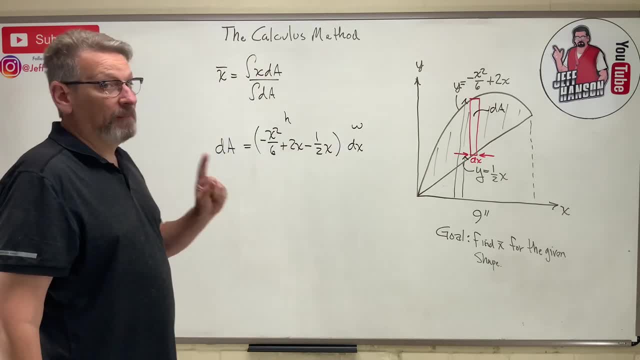 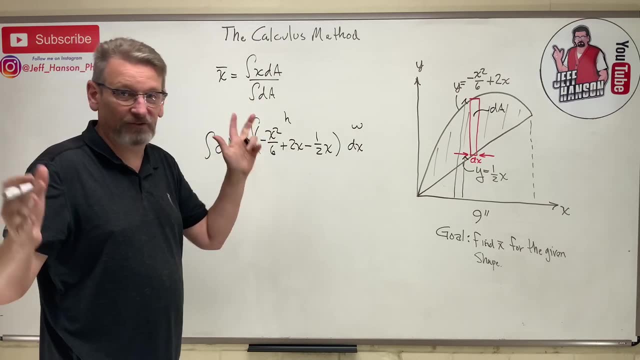 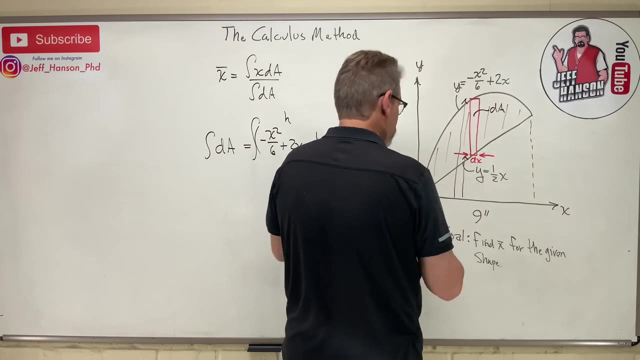 just d x. Okay Now, remember when we integrate, because we need the integral of d a, so we need the integral of all this. But when we integrate, we have to have limits. And where's our stack of strips? our stack of books goes from zero over to nine. This is nine inches. Okay Now. 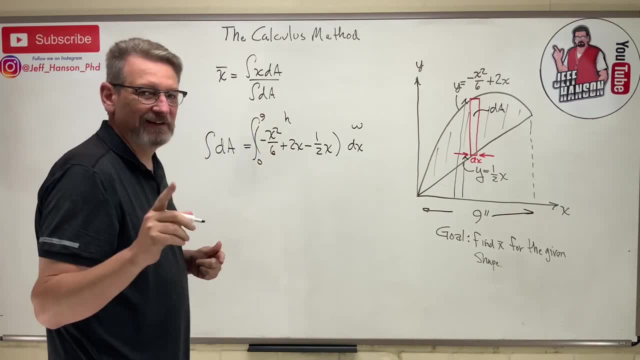 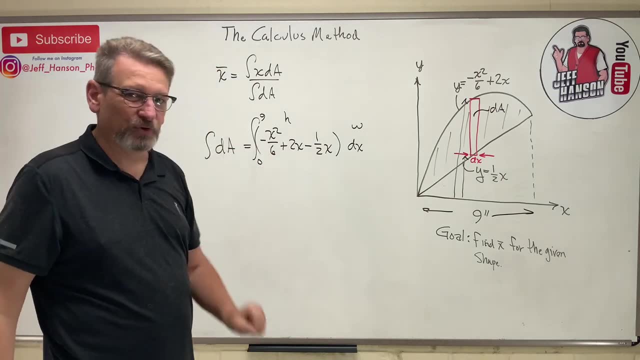 I'll tell you this- I shouldn't tell you this, but I'm going to tell you this- Your TI-36 pro calculator. you can just enter that into it and give it the limits and it'll do it for you. Okay, it will do. 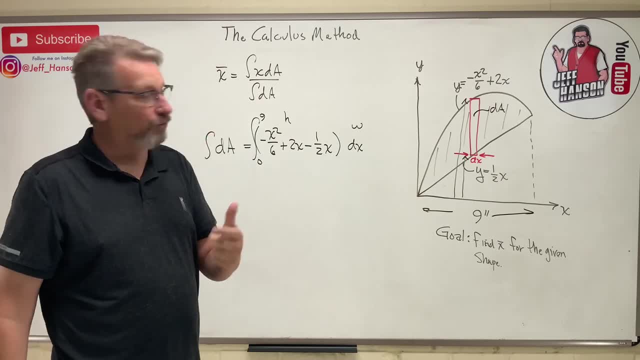 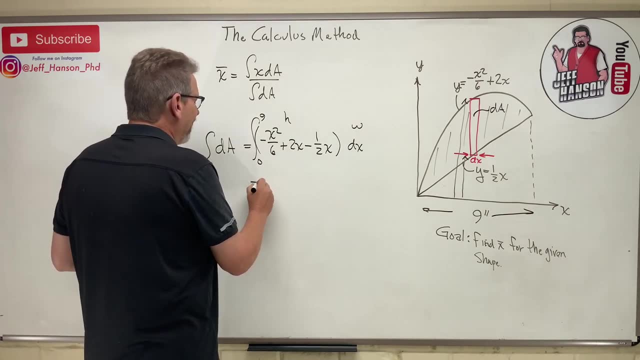 integrals for you. Yes, a solar calculator will do integrals for you. I'm going to do it by hand for you And let's see what we get. Okay, So I get minus one. sixth, I'm pulling out. I like to pull. 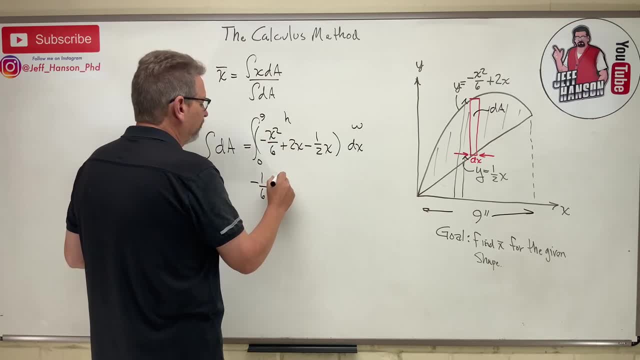 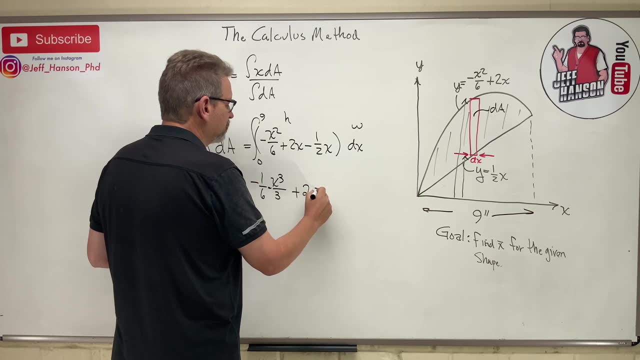 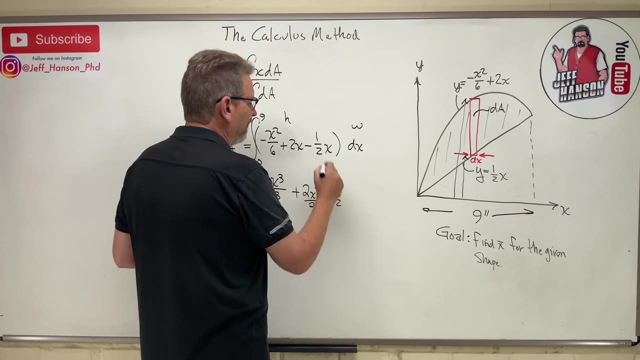 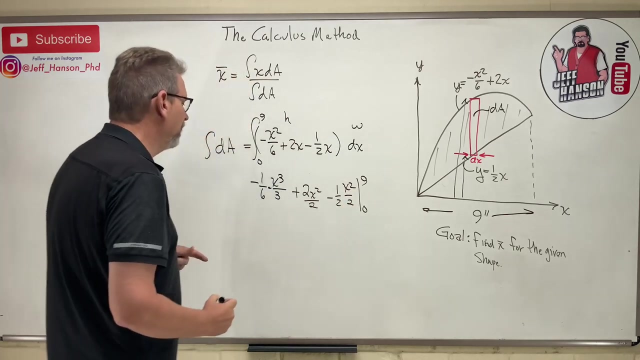 out the constants, right, And that leaves me with x squared, which becomes x cubed Over three. plus two. x becomes two. x squared over two, Okay, And then minus, that's one, half is the constant. and then x becomes x squared over two. from zero to nine, Okay, And so this becomes. 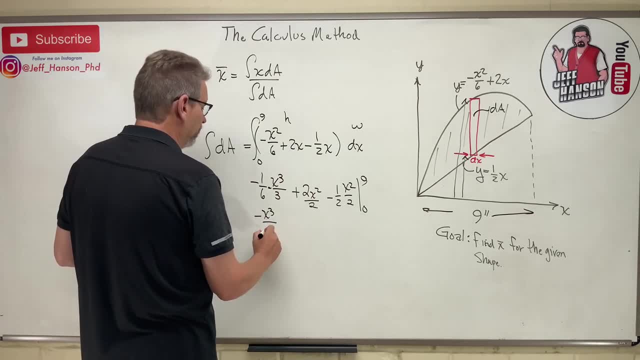 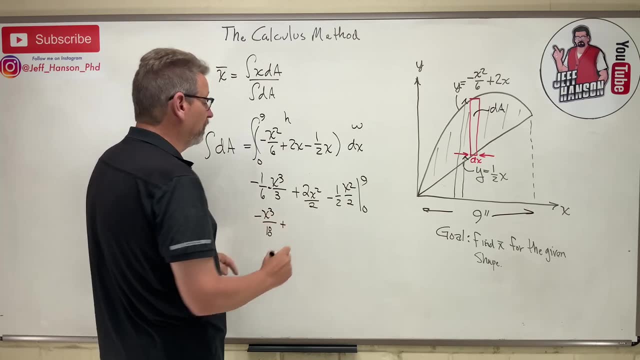 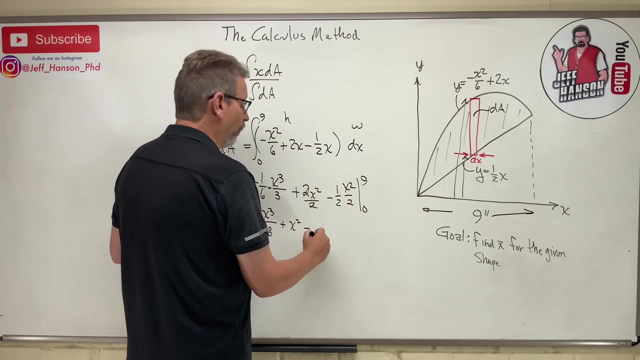 negative, x cubed over 18.. Plus what Two? oh that, just those cancel out, don't they? Plus x squared minus, what does that become One? fourth? no sorry, x squared over four, right, Minus x squared over four. Well, that's a fourth. 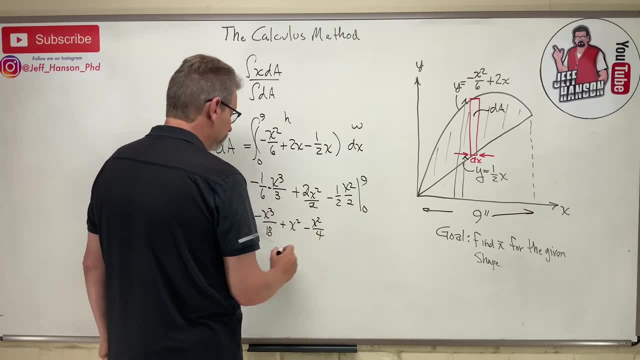 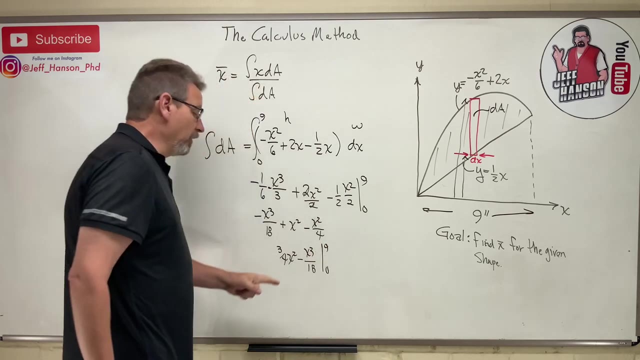 of an x squared off of a whole x squared leaves three fourths of an x squared, doesn't it? Three fourths of an x squared, minus x cubed over 18.. Okay, And then that's from zero to nine. So everywhere I have an. 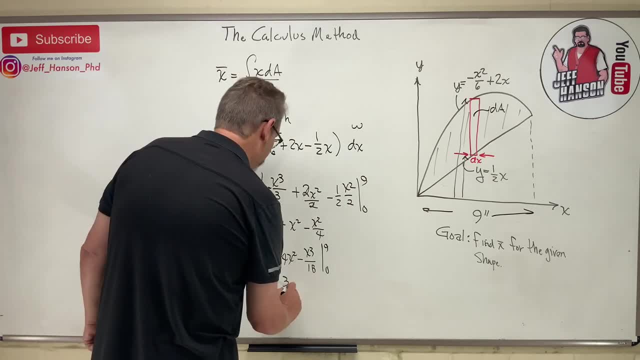 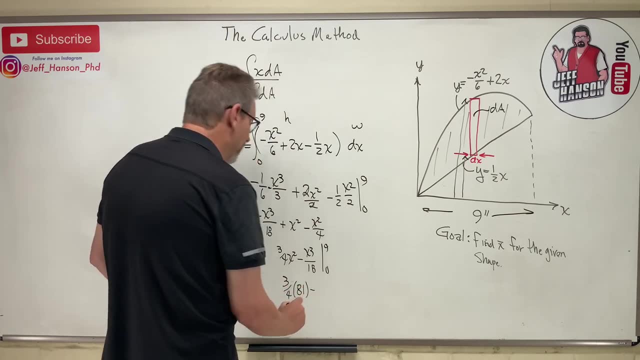 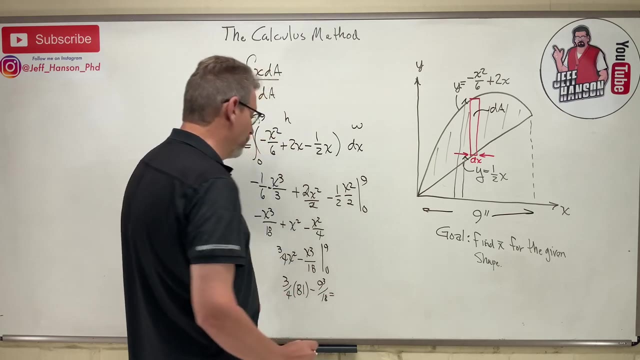 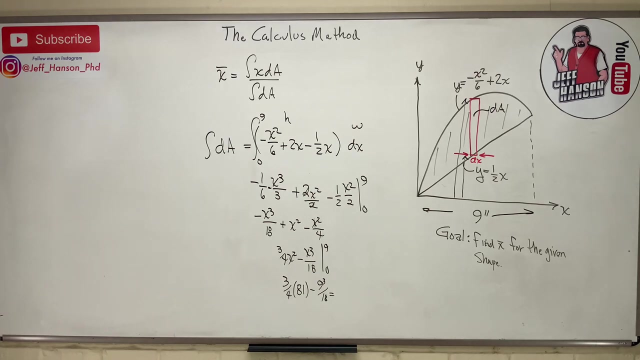 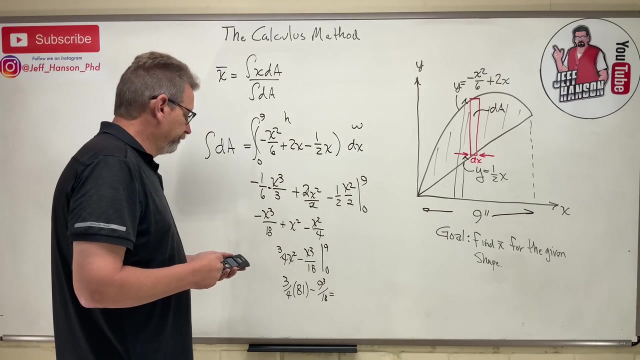 x. now I just plug in a nine, So I get three fourths of that's 81, right Minus nine cubed over 18.. And so that gives me minus divide a nine. now I get a nine. Next, I just plug in a three fourths of whatever. 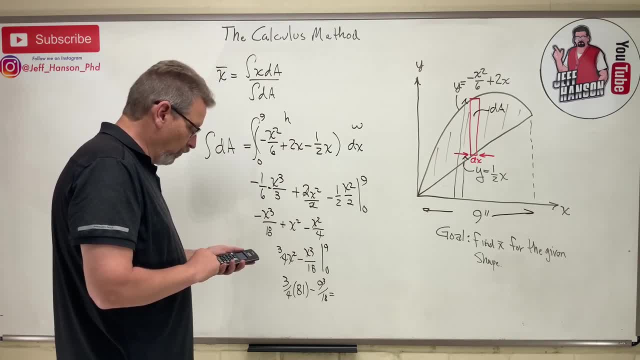 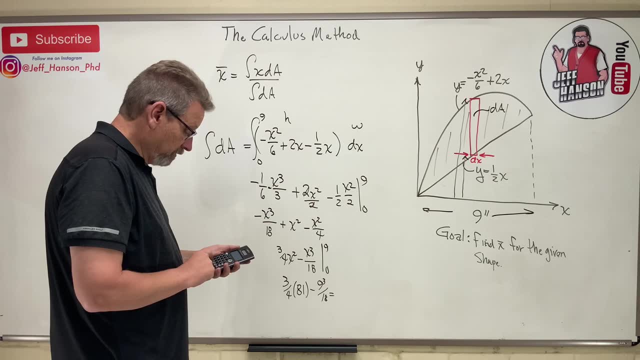 am I doing here? theta four squared over capital X. Honda squared of x squared over the negative x squared over ten people on my measuring board. Let's do this. I get a plus three, four. thee cubed x squared over. let me do it again with this theta four squared over. let me do it again with this theta four squared of x squared over nine. I take that, I take that twice and I butt: vemos el menos la opinio es x cuadrado por día. posture. 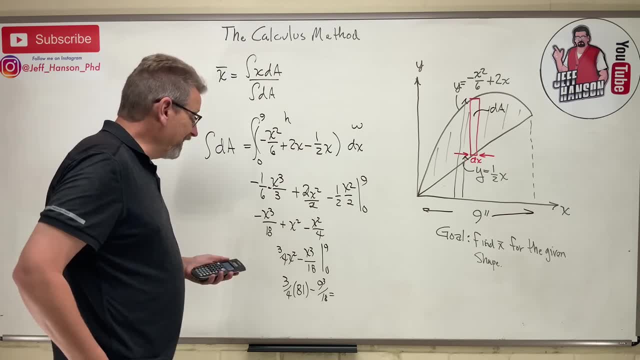 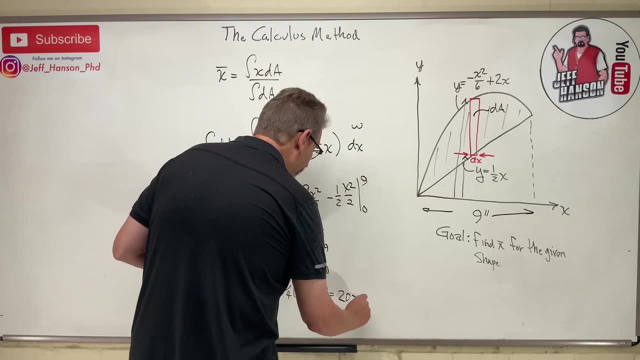 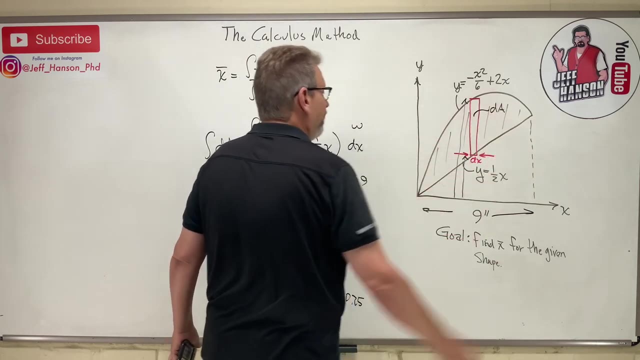 Minus um. what Nine cubed divided byane When cultiv EPA homeWhat Nine cubed divided byane- 20.25. and so what is 20.25?? Well, I'll tell you, 20.25 is the entire area of that shape. 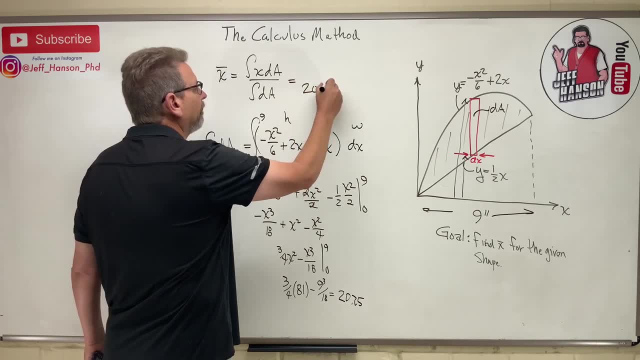 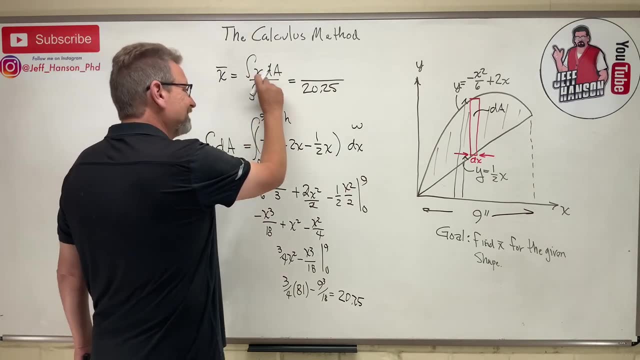 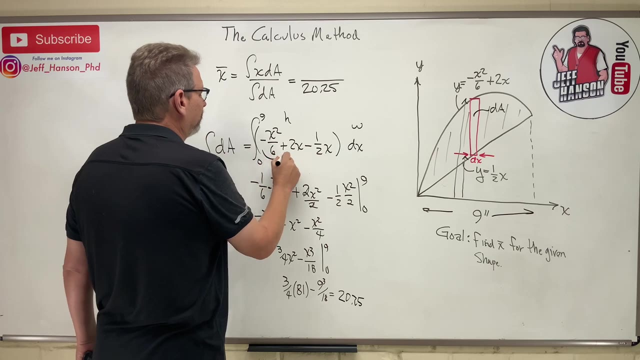 and that goes here. What goes on the top? Well, that's x times dA, unintegrated dA. What is unintegrated dA? Well, unintegrated dA, is this business right here, isn't it? So you know what? 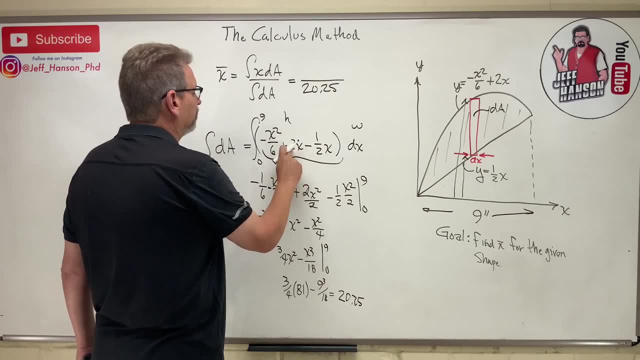 Let's fix this: 2 minus 1 half is what 3 halves, right? I'm just simplifying a little bit, just simplifying with a little algebra. So let's take unintegrated dA and multiply it times x. 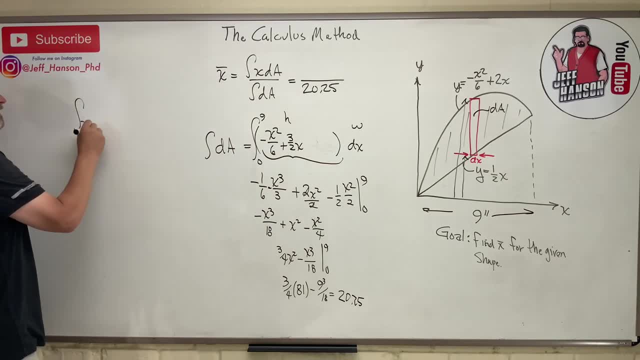 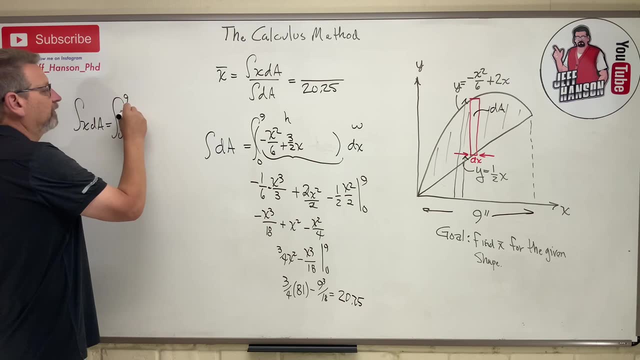 And I get this. The integral of x- dA is equal to the integral same limits. Now I'm going to multiply x through, and so I get minus x cubed over 6 plus 3 halves x squared dx. Let's integrate this. 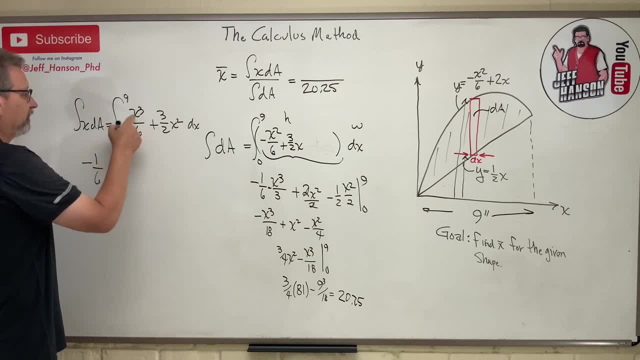 So we get what Negative: 1 sixth x cubed becomes x to the fourth over 4.. And then plus there's my constant 3, 3 halves and x squared becomes x cubed over 3.. Those 3's cancel out. 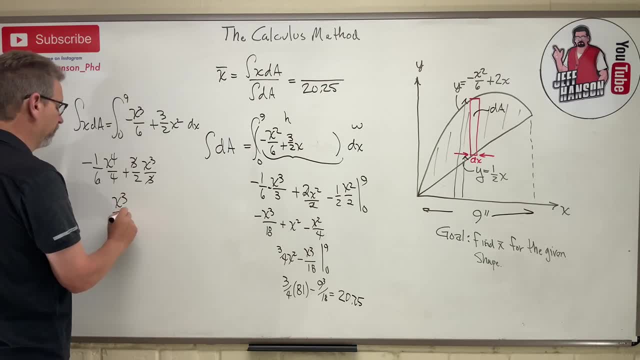 So I get, uh What do I get? x cubed over 2 minus x to the fourth over 24 from 0 to 9.. So I get 81 over 2 minus 9 to the fourth over 3.. Alright,